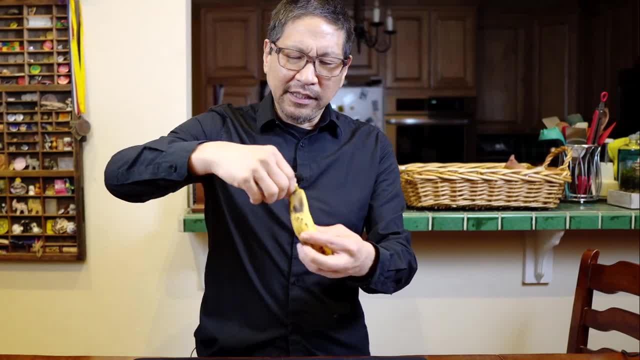 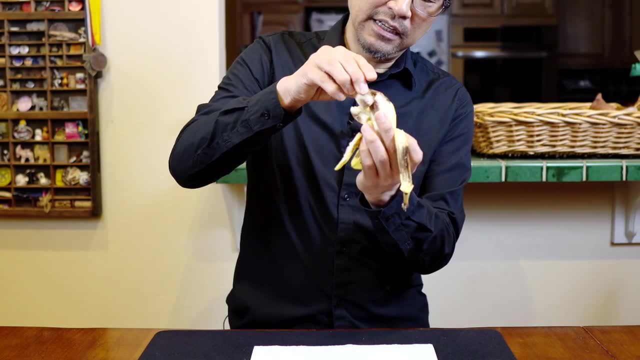 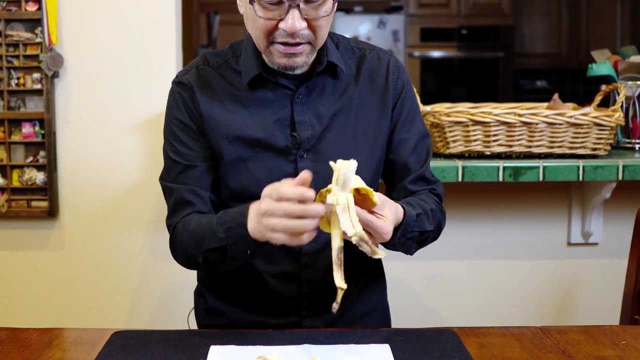 A banana inside of its peel. If I have accomplished this, it's either magic or a little trickery, but let's peel the banana away And, as you can see, there's one slice there and another slice there and another slice there. 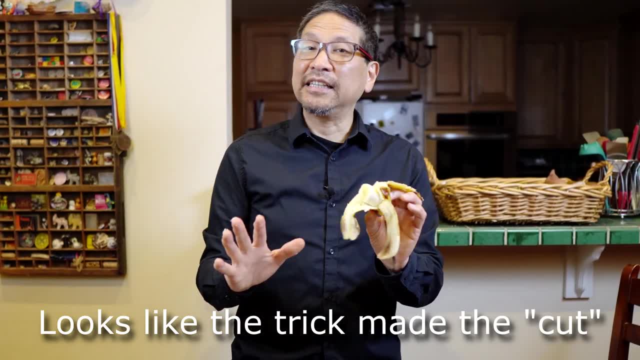 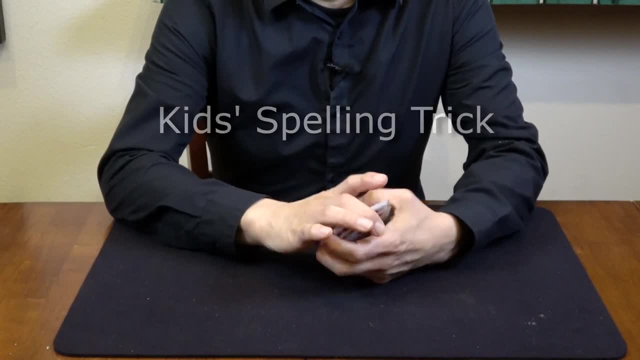 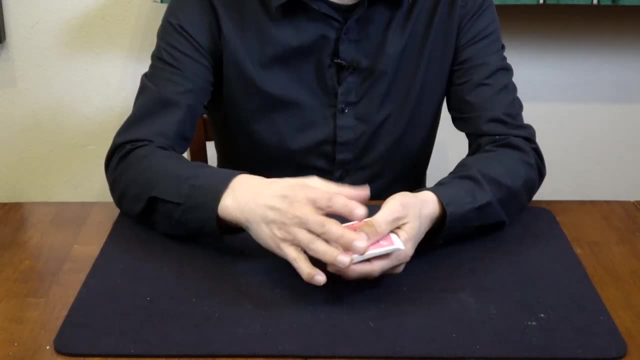 The banana has peeled inside of its peel. I have here some cards and we're just going to spell and see if we can go to every card. So we're going to start at the bottom with an ace, So let's spell ace A. 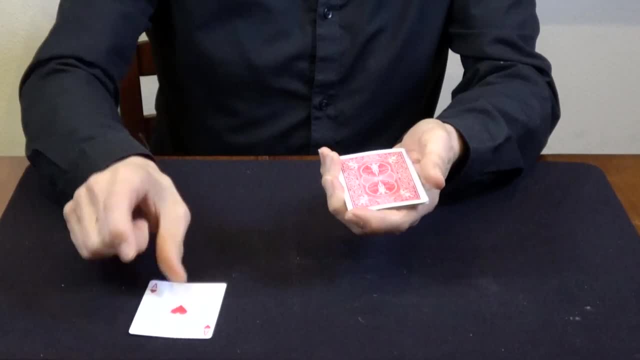 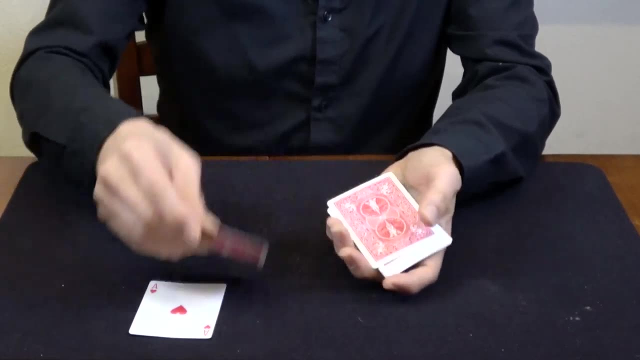 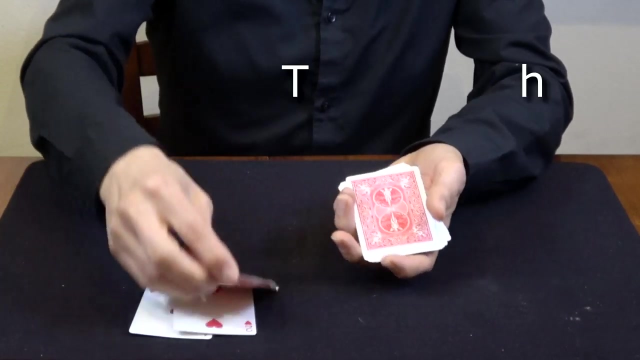 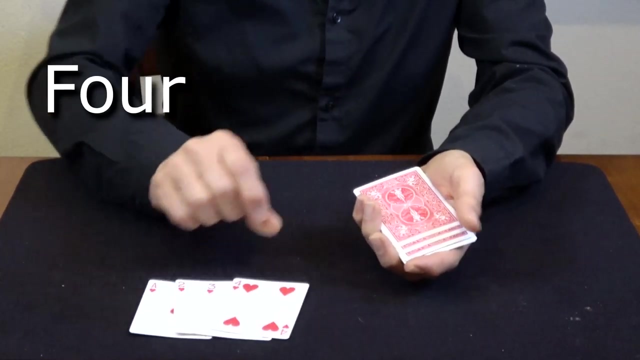 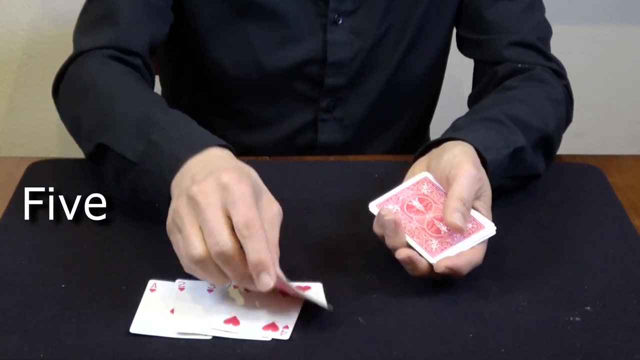 C E and that should bring up an ace Two T W O, Two Three T H R E E, Three, Four F O U R, Four, Five F I V E, Five, Six S I X, Six, Seven. 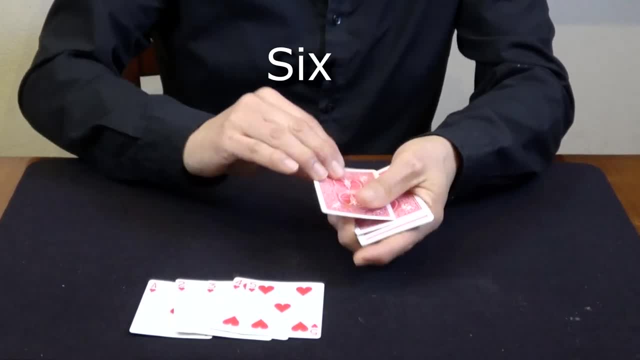 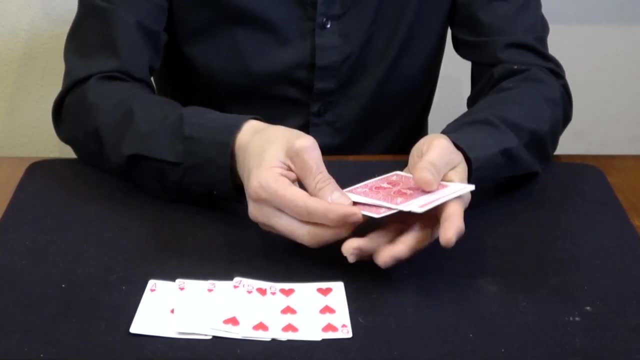 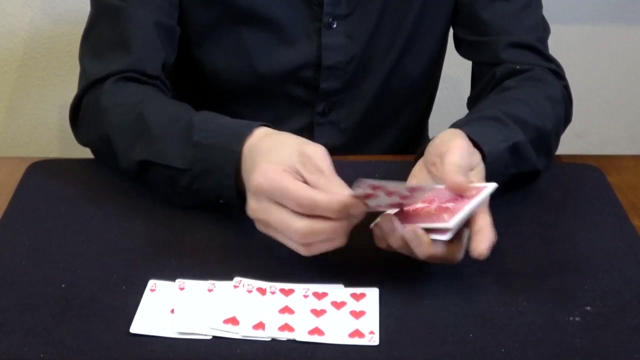 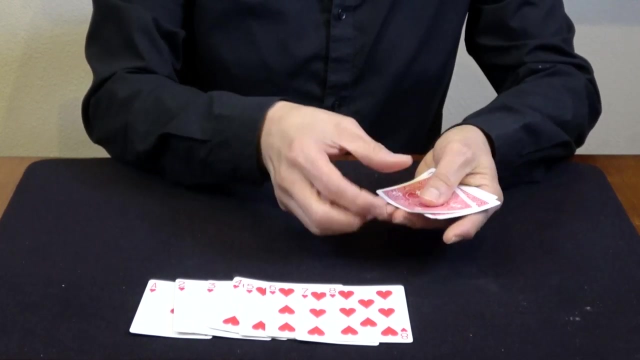 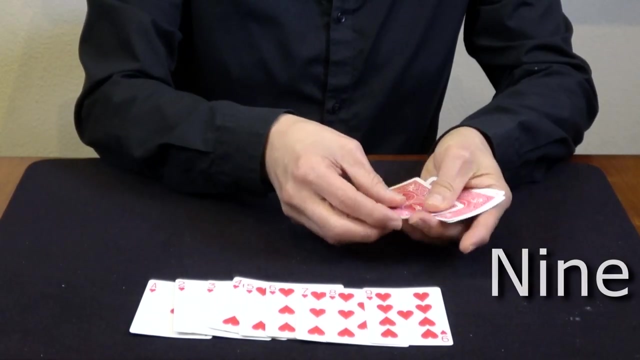 S E O Three T H R E E Three T H R E E V E N N. 7, 8 E I G H, T, 8, 9, N I N E, 9 T E N 10, Jack, J, A, C, C J. 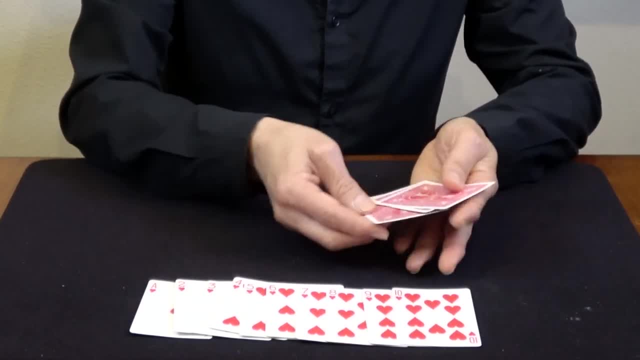 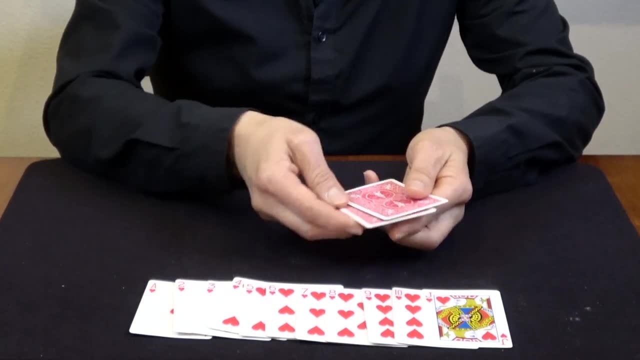 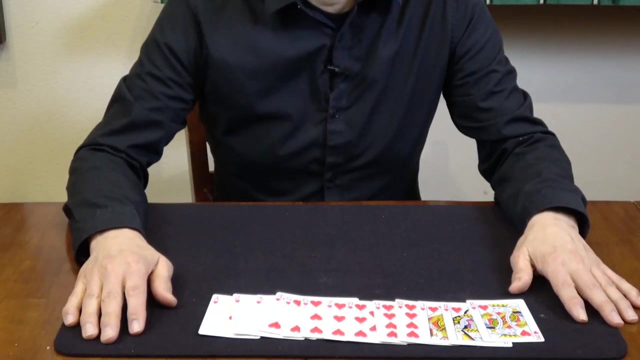 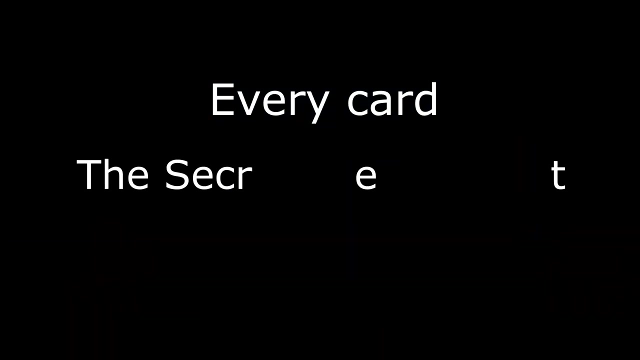 A, C, T, T, J, J, J A, T, M T, K, K, J, Q, J E N T T E N, Q, Q E E N, Queen And The King. And there we've done it. We've spelled to every card, One by one. So here's how you perform the floating Jack card. 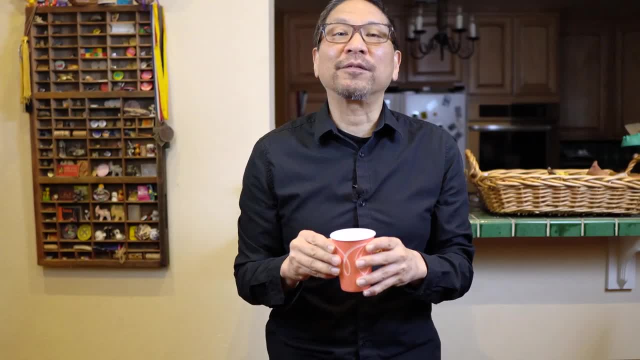 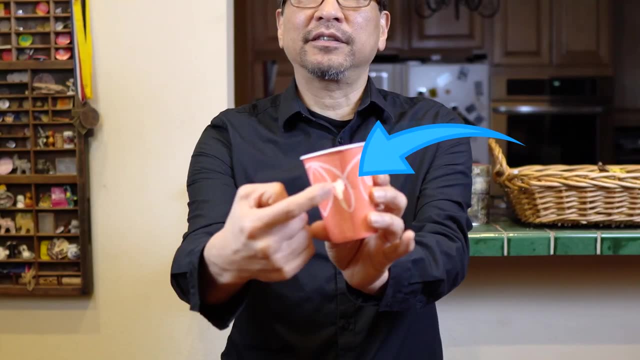 The magic trick is to use a card called the card of the card. This card is called the card of the card, So here's how you perform the floating Jack card. The card of the card is the card of the card cup. What you're going to need is a paper cup, and beforehand you punch a little hole in the cup. 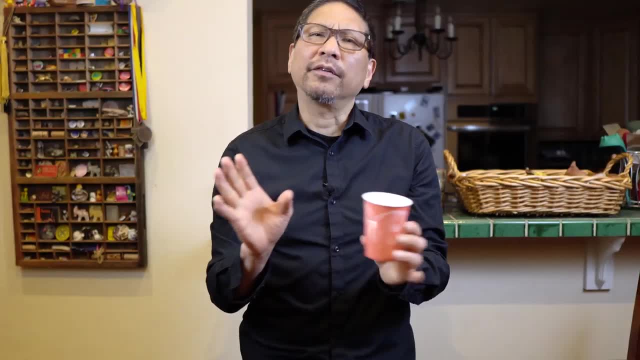 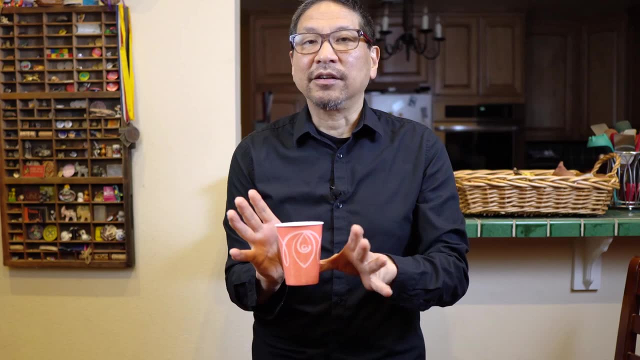 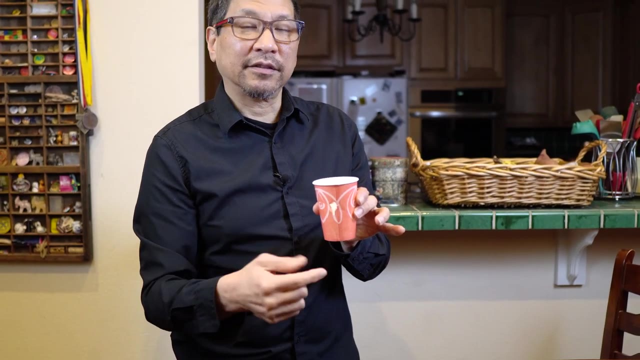 right here, and that's where your thumb goes in. If you look back at the performance footage, you'll notice that you don't see my thumb because you can't perform the trick like this, So all you do is insert your thumb into the hole. You probably need a grown-up to use a pair of scissors to kind. 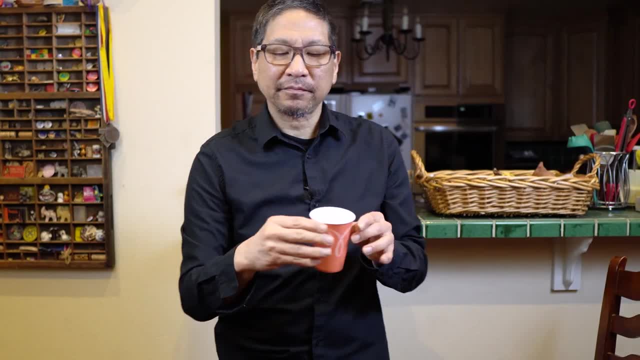 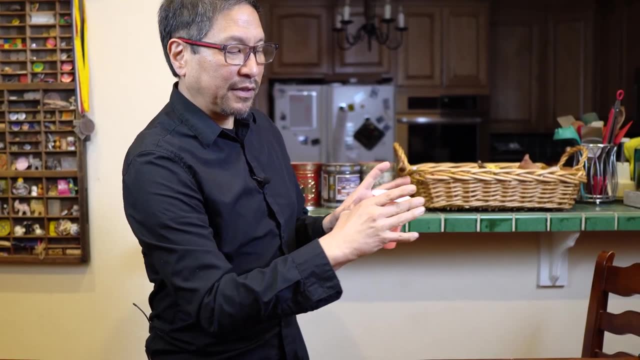 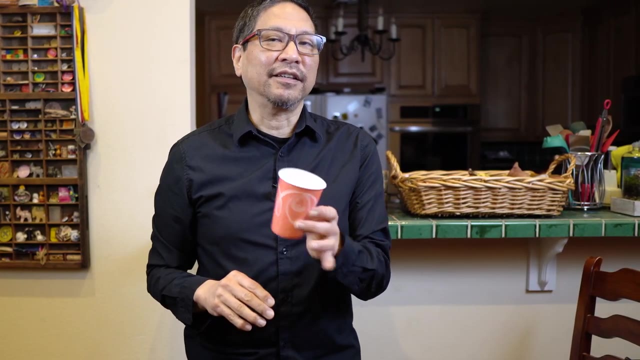 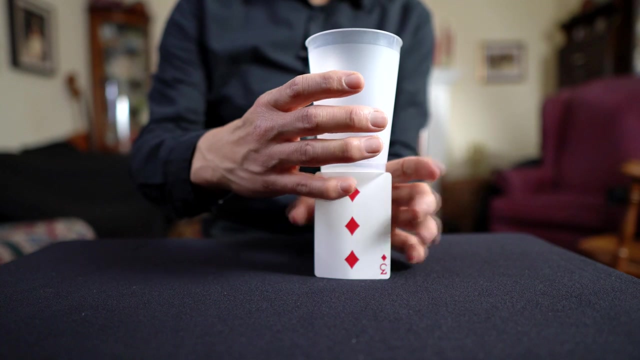 of cut this out, but just enough to hold your thumb. and then, here, all I'm doing is just letting go of my fingers and wiggling them a little bit and creating that effect as if the cup is floating. and that's the floating cup For your gimmick. you're going to need two playing cards. 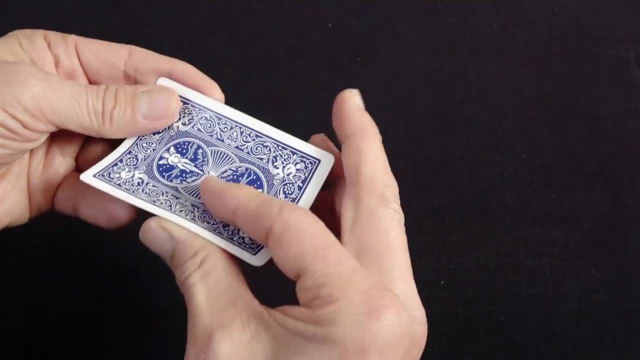 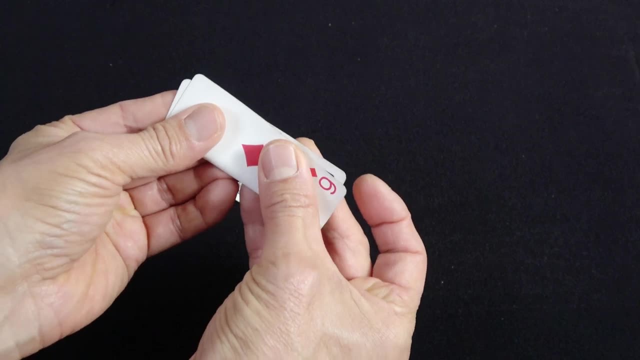 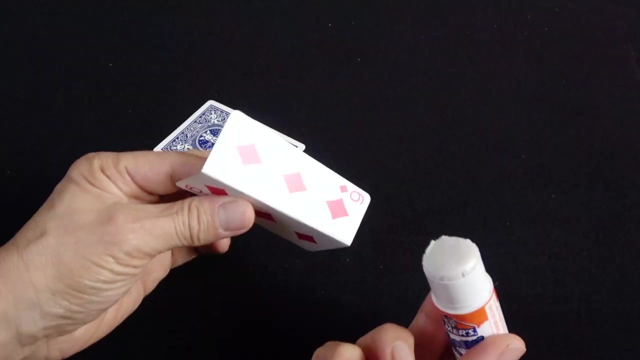 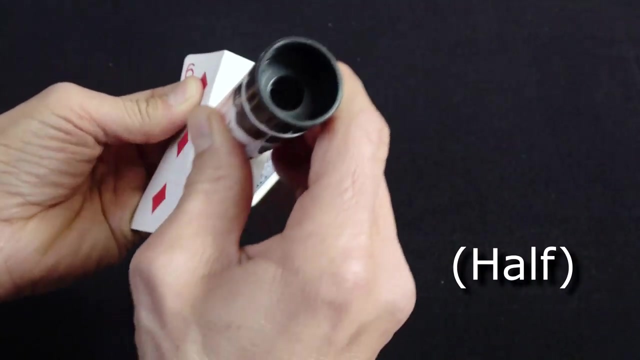 Take one of the cards and fold it in half this way lengthwise, but what I want you to do is not fold it straight, but fold it at a slight angle, just like that. This will assist you later when you perform the trick. Take some glue and place it on half of the card. 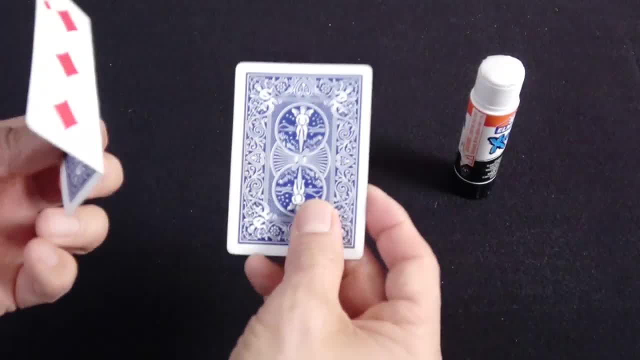 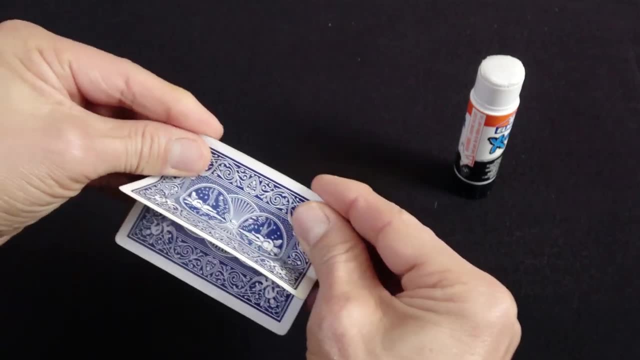 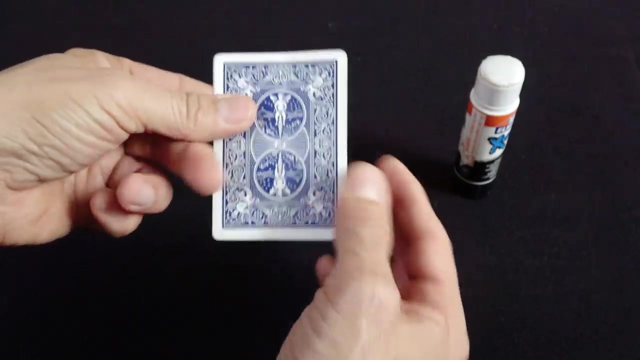 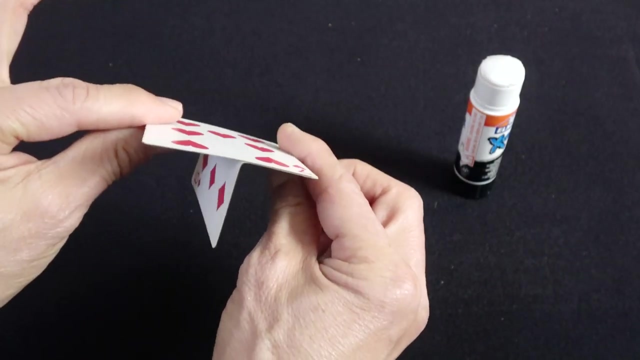 and now you're going to simply fold, glue this half onto the other playing card, Line it up on one side and you'll have a card. that looks fairly normal when you hold it like this, but when you need to, you can open this up and it creates a flap, which is the secret to 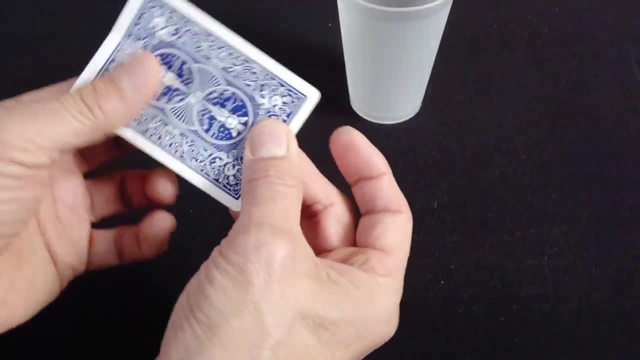 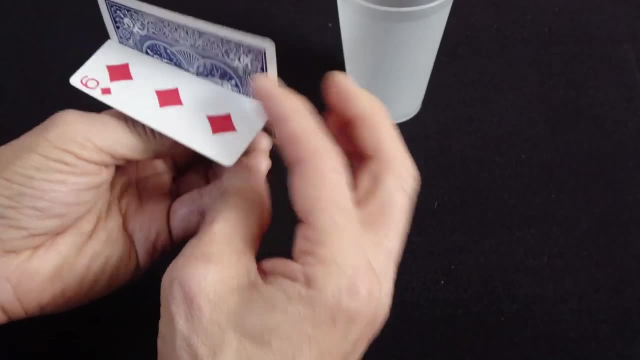 the trick. Now let's talk a little bit about performing the trick Now. when I had you make the gimmick, I asked you to fold the card in an oblique, off-center manner, and the reason why is that the longer edge here will work to your 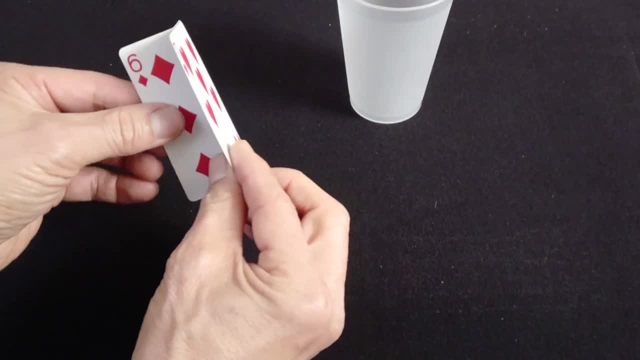 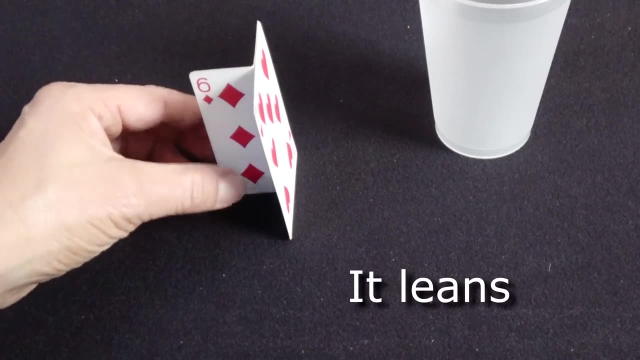 advantage? First of all, it's a little more stable because it's longer. Second part is it's actually a little shorter than the front, and that allows the card to lean back just a little bit, which assists with the trick. So here's how to. 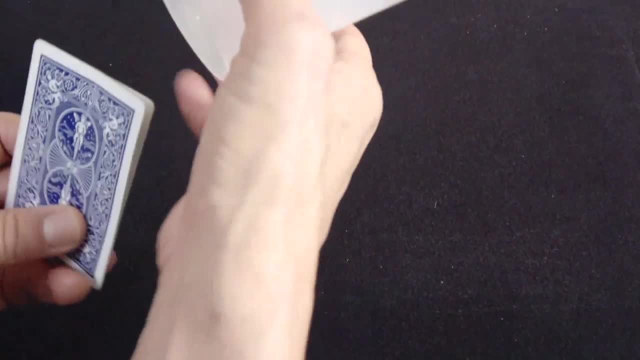 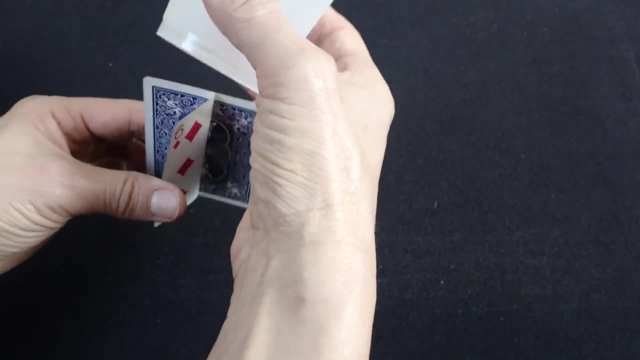 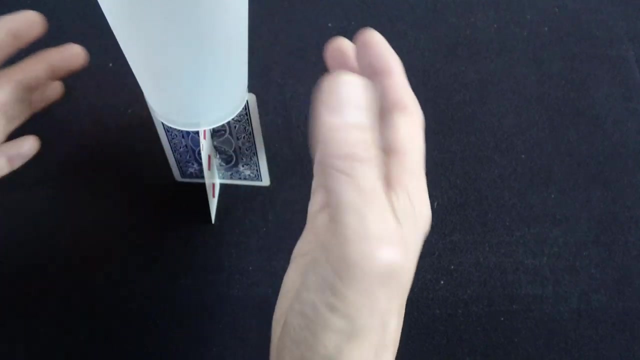 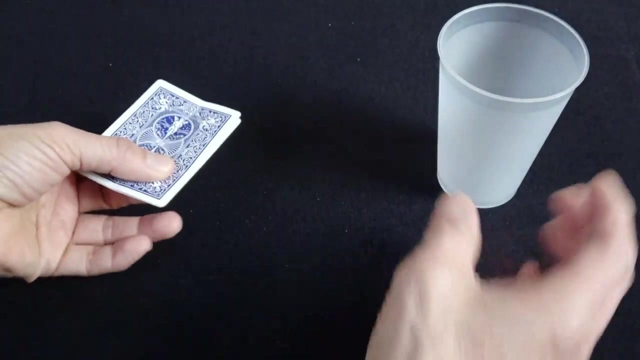 perform the trick. You can show the card and then you show the cup. and as you show the cup, take the card and fold it in half. Your finger, thumb fingers and thumb rest the cup on top and you'll find that it balances. and to end the trick, show the card and the cup. 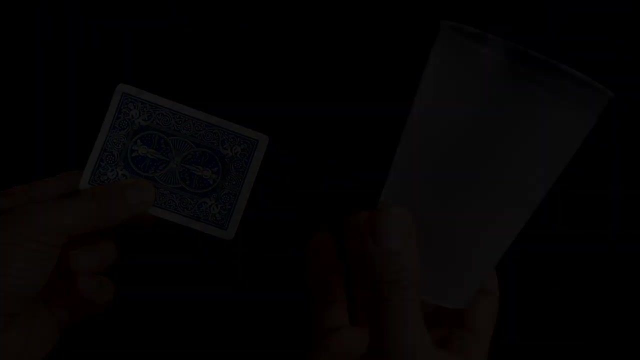 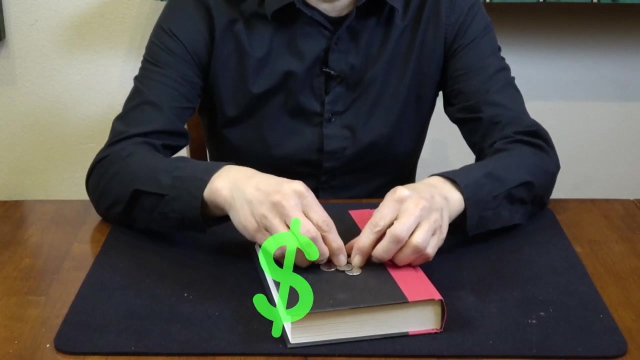 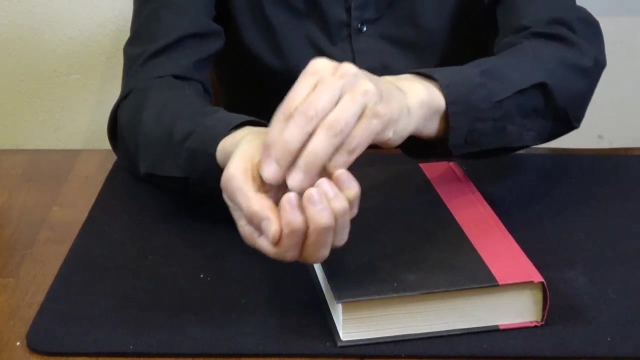 That's the cup on card. So here's how you perform the trick. Now I'm going to show you how to do the trick. You're going to have to start off by multiplying coins in a book. Now you'll notice here that I have first 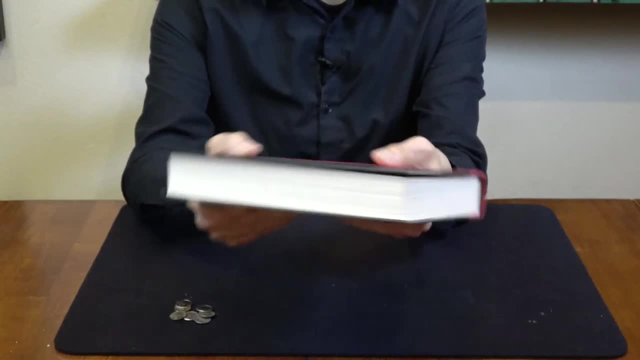 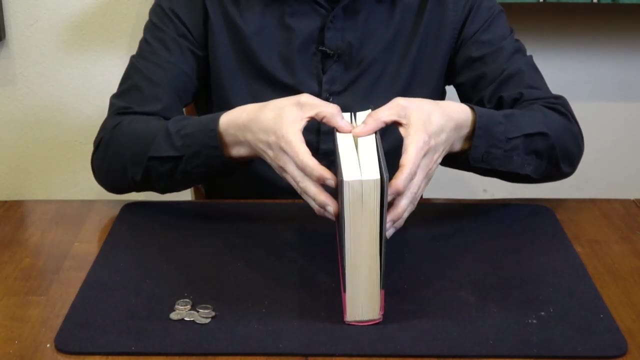 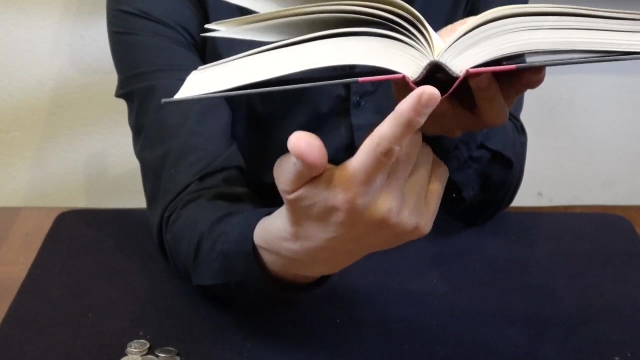 of all coins. I think I have seven here And I have here a hard back book which is how this thing works. Now, before you do the trick or you walk out and see your audience, you take the book you want. You see, right here There's an opening in the binding. That's the secret to this trick. 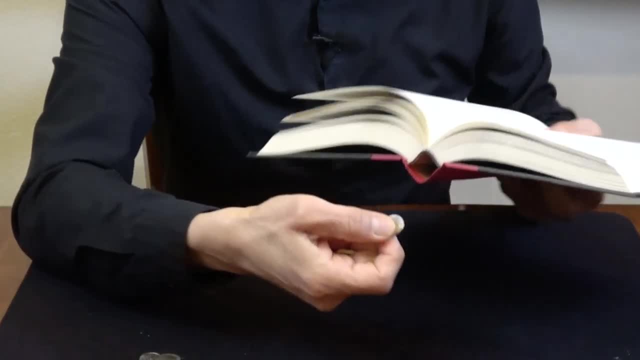 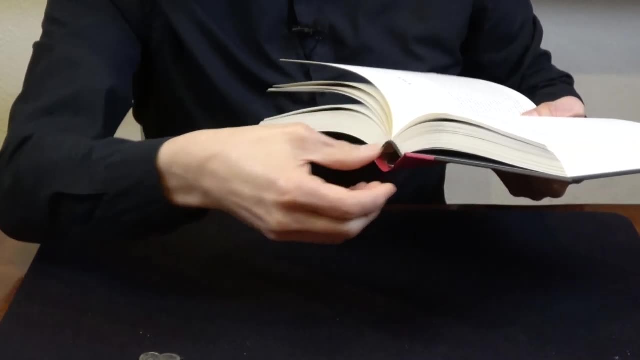 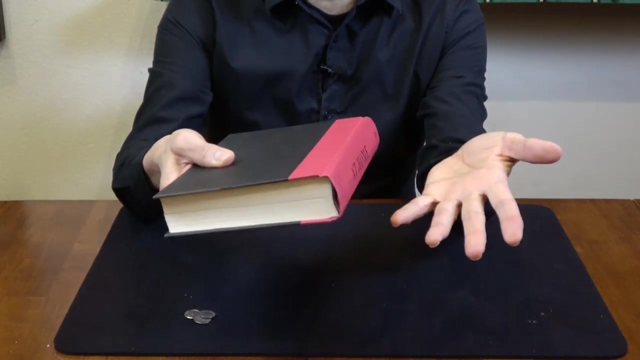 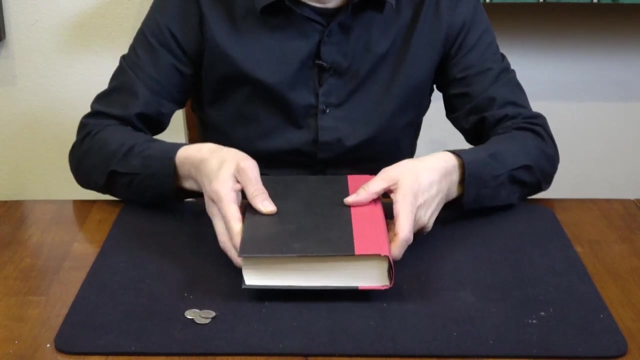 So beforehand you take some extra coins and you just insert them into the binding of the book, Close the book up and Because of the way books are designed it actually holds those coins in place fairly nicely. So you walk out and you say: I'm going to show you a trick with this book here. 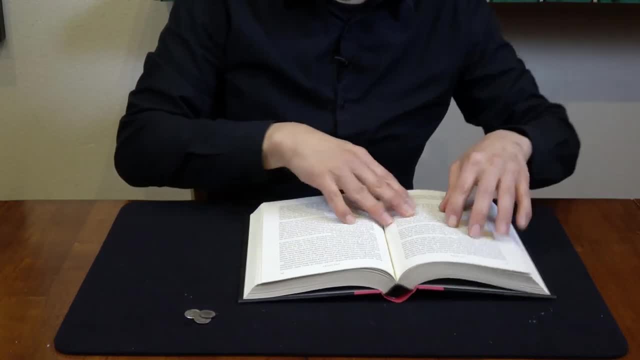 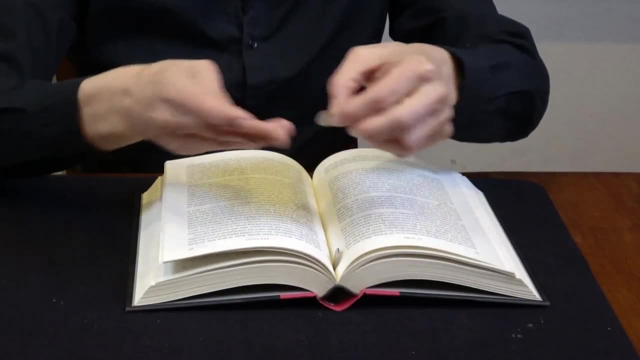 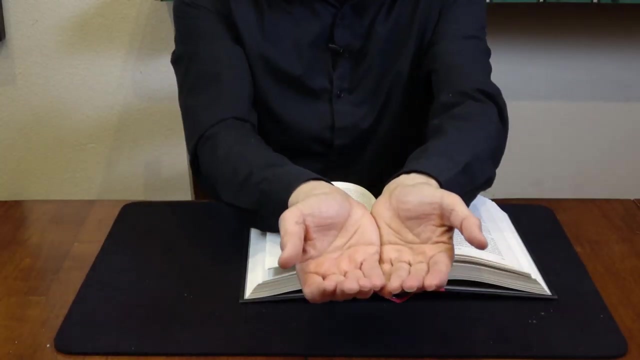 Just so I keep the coins out of my hands. I'm gonna give these to the spectator. You have the spectator take the coins and they count the coins: one, two, three. make sure they clearly count the coins and then, if you like, you can dump the coins into your hand or have the 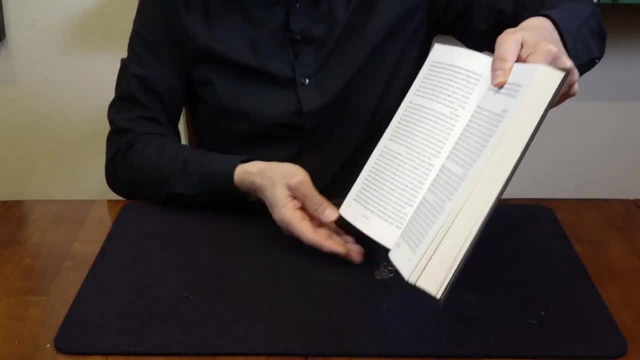 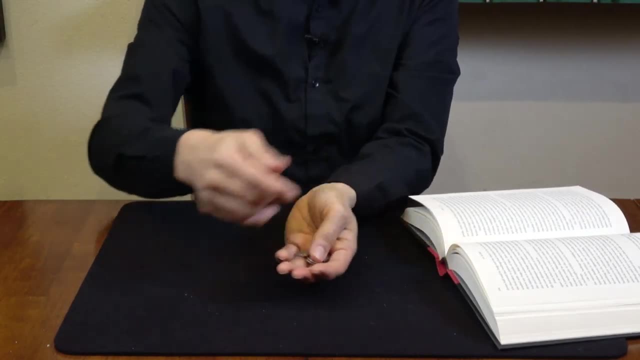 spectators hold out their hands. but When you dump out the coins- Hopefully a little neater than that- You'll see that the other coins from inside of the book binding come out and you'll have seven coins where formerly there were three. a multiplying coin trick. 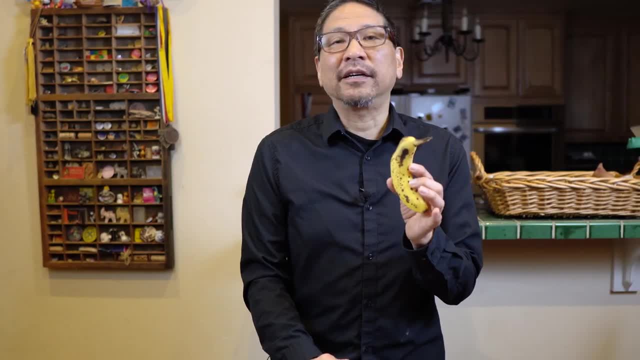 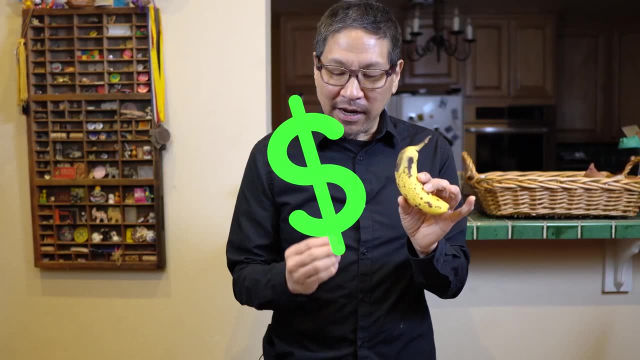 Here's a trick with a banana that you can do. it's kind of fun. sorry, I don't have a better-looking banana. We're kind of a limited budget here, but what you're going to do beforehand is take your banana and you're gonna need a. 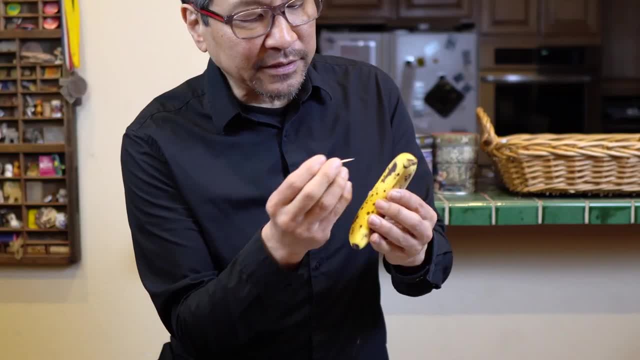 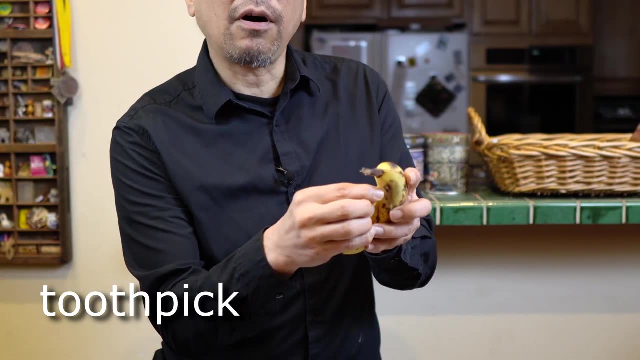 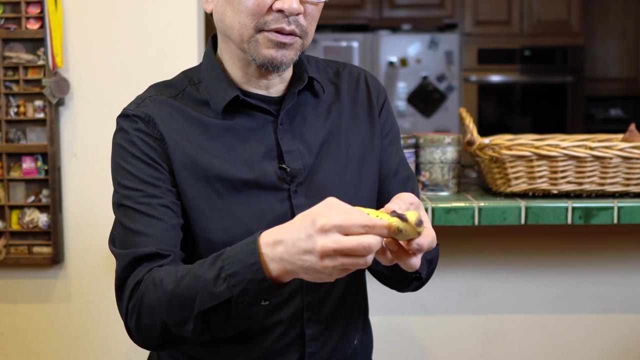 toothpick. so what you're going to do is Using the toothpick. you're going to just poke the toothpick into the banana Now, don't go all the way to the other side, But then you just move this toothpick back and forth and essentially what you're doing is you're slicing. 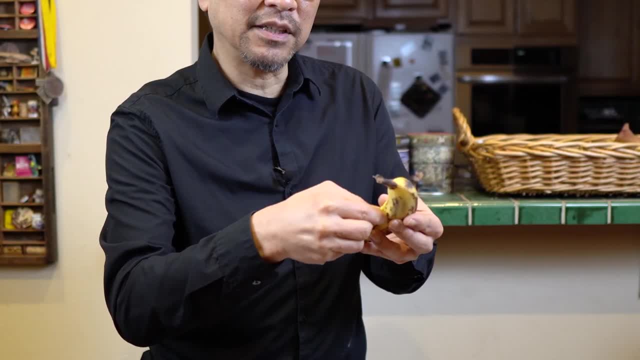 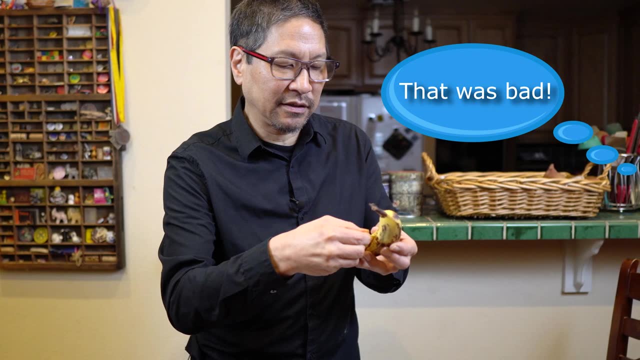 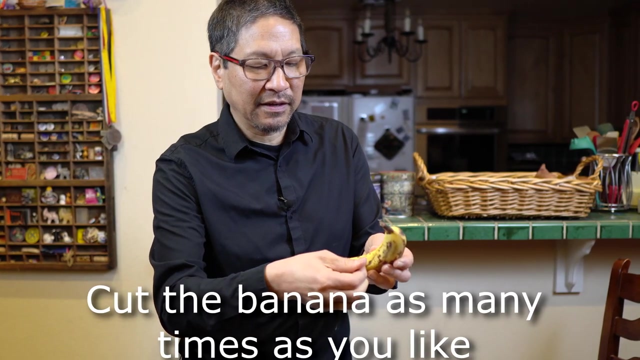 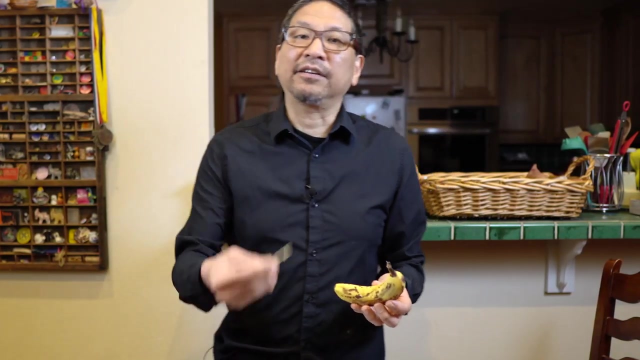 the banana inside of its peel. Okay, I got to say it. this is an appealing trick. I'm going to show you how to do it. All right, let me just do one more here So you can see how it looks And you get rid of the toothpick. but now you're ready to perform the trick? 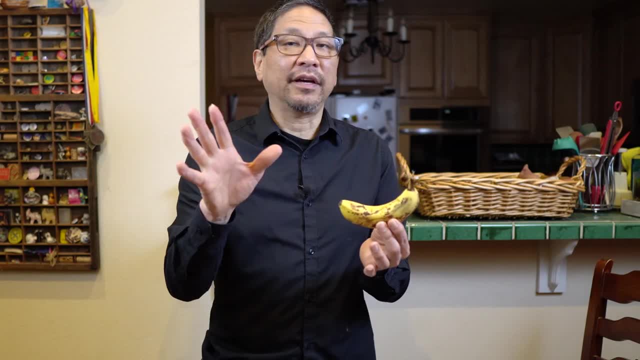 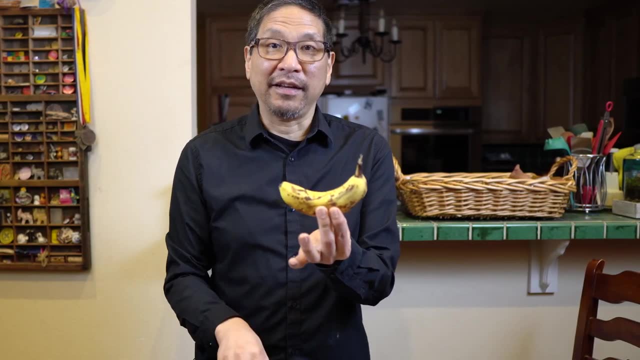 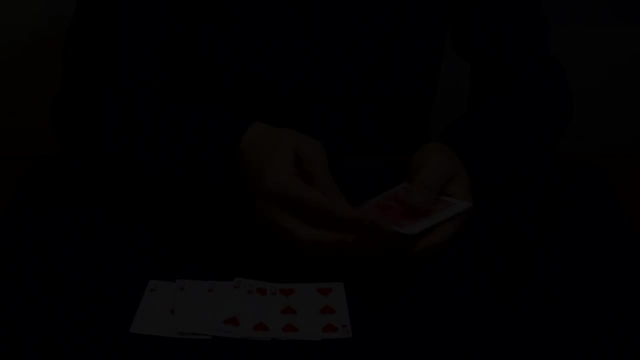 So all you do is just come out, show your banana and then create whatever theme you want to do, And then, when you peel the banana, The slices will already be made inside. Here's how you perform the trick. Here's how you perform the trick. you're going to need the cards in a specific order, and 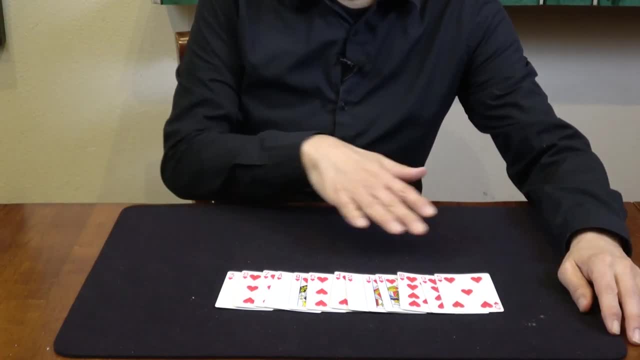 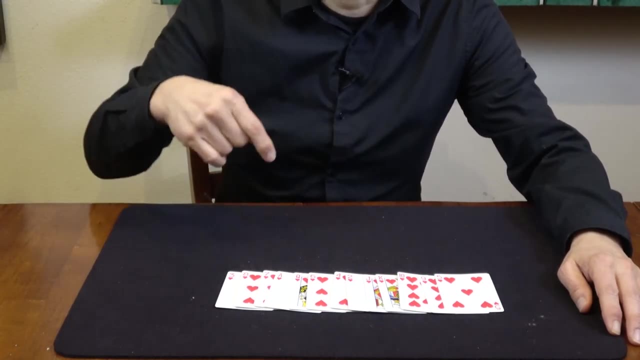 That's the secret, And so here's the order here: Just take out the ace through king of one suit, line them up this way. I'll put this on the screen as well as inside The description for this video. but you have your three, eight, seven ace. 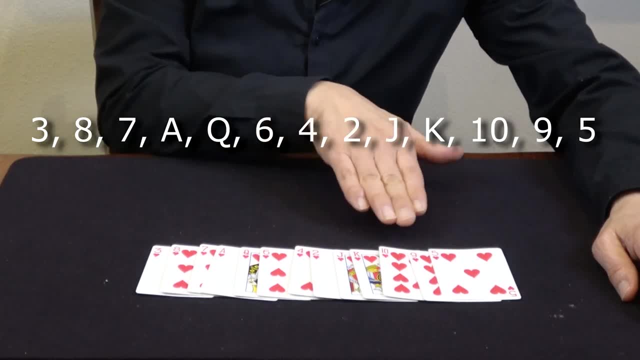 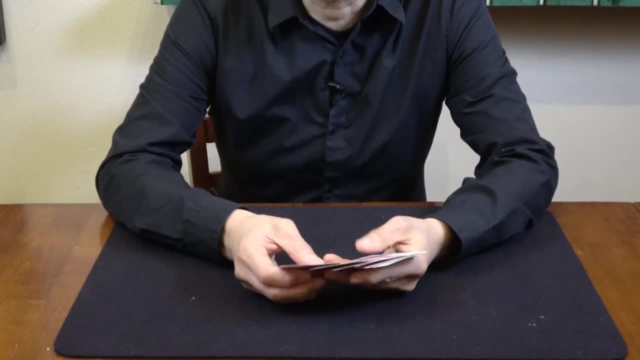 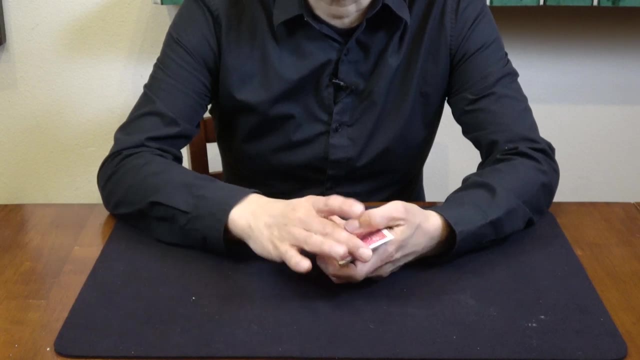 Queen six, four, two, jack king Ten, nine and five, and you're ready to perform the trick, just as I did. inside of the performance, All you're doing is spelling each card in order A-C-E for ace. you put each card on the bottom and then the next card is the one that gets turned over. 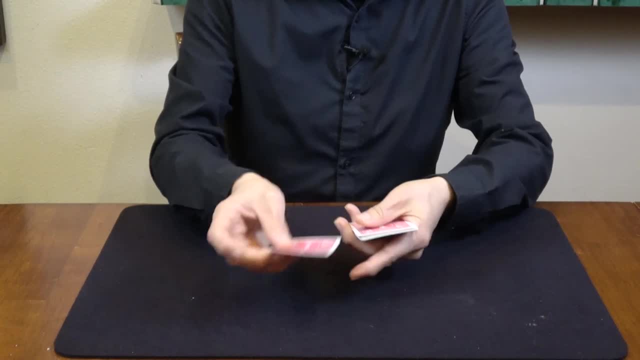 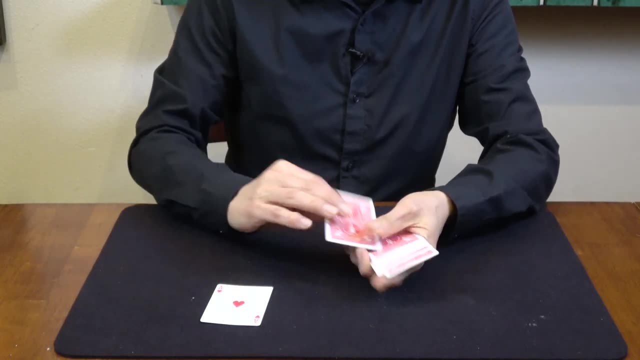 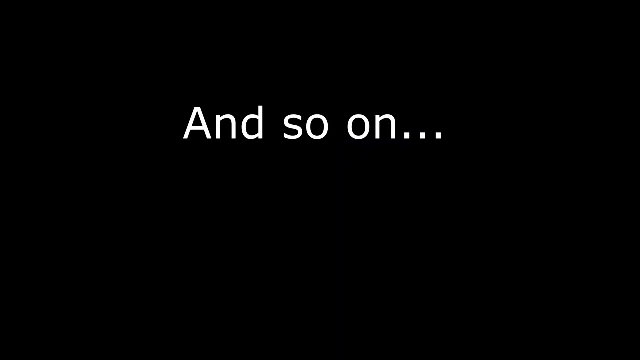 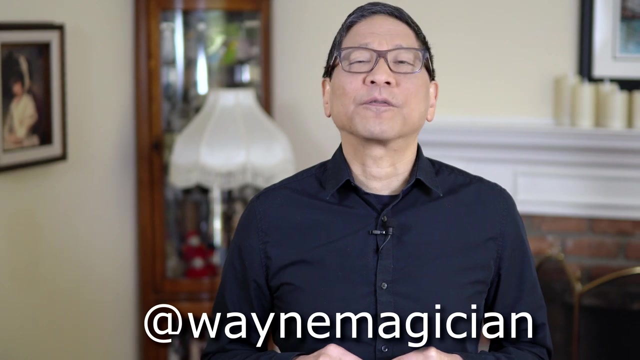 So let's try that here. So I'm gonna go a C-E and that should be an ace T-W-O, and that should be two: T-A-C-E, H-R-E-E, three. Well, I hope you have fun performing these easy magic tricks for your friends and family. 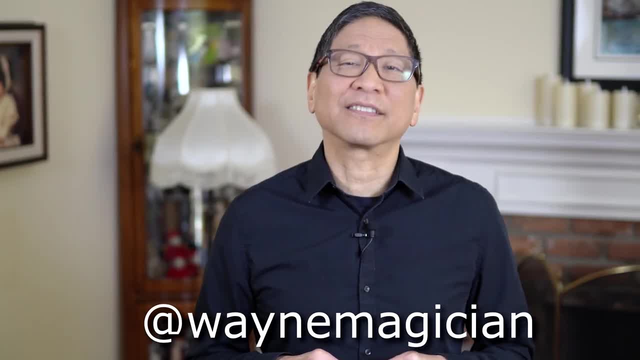 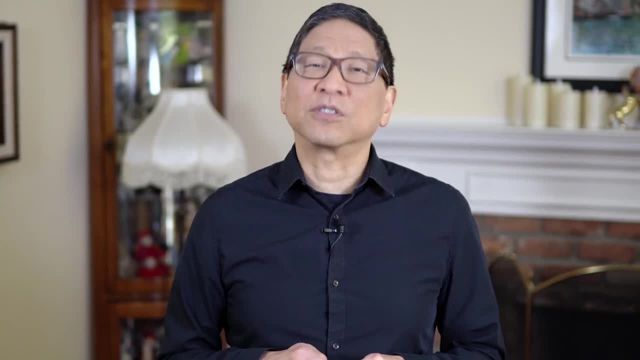 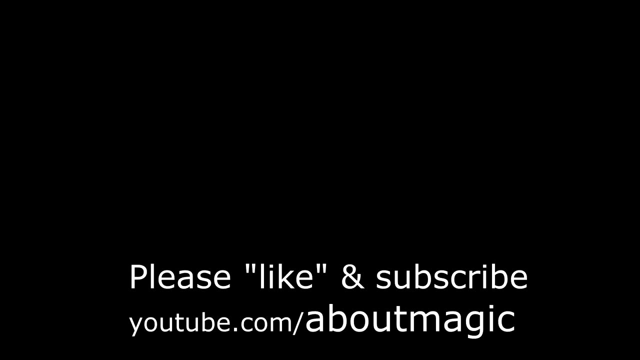 Please give us a like and please subscribe for more video lessons in the future. And, by the way, please comment below if there are any tricks that you would like us to teach in future lessons. Thank you for watching. See you next time, You, You.